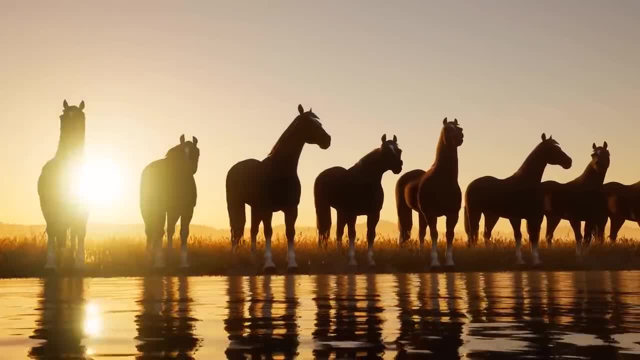 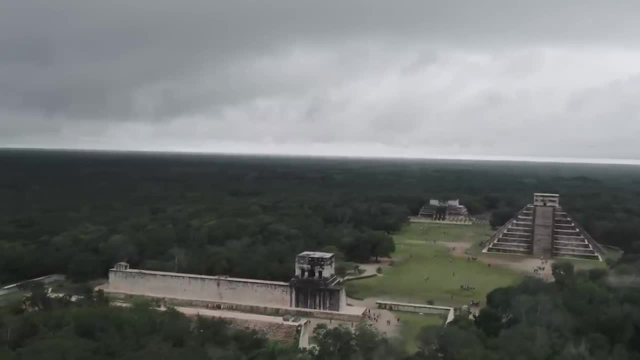 stretching thousands of miles across the Eurasian landmass to connect China with Europe. but nothing comparable was possible in the Western Hemisphere to connect the Iroquois on the Atlantic seaboard of North America with the Aztecs of Central America. Italians could. 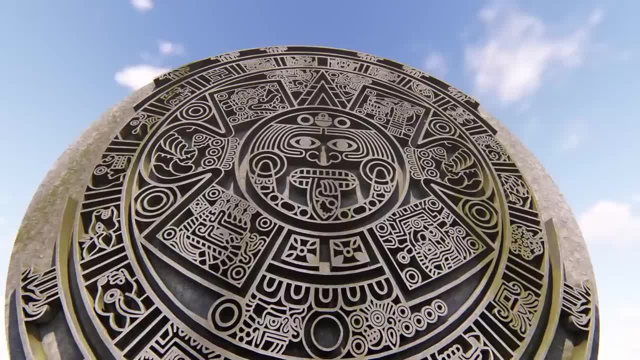 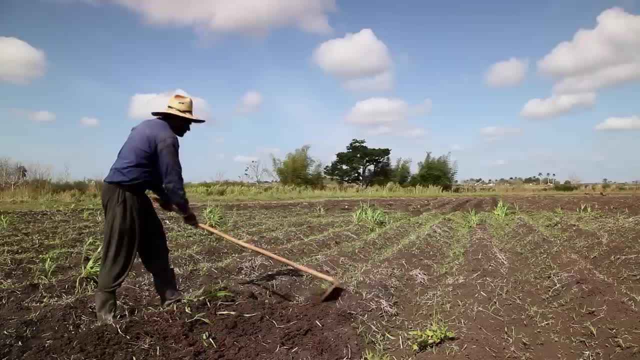 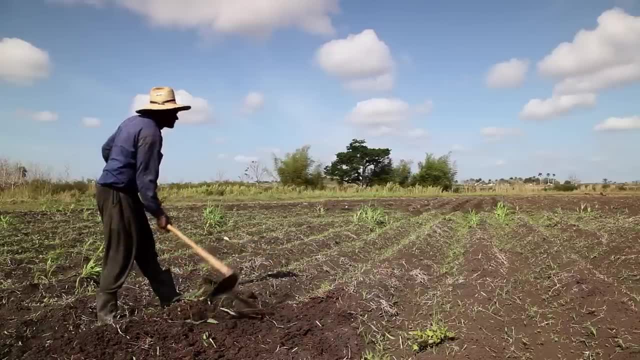 acquire spaghetti from China, but the Iroquois could acquire nothing from the Aztecs, or even be aware of their existence. Agriculture in the Western Hemisphere was inherently limited to what could be accomplished without animal muscle power: to carry or to pull loads, or to plow the land as well as. 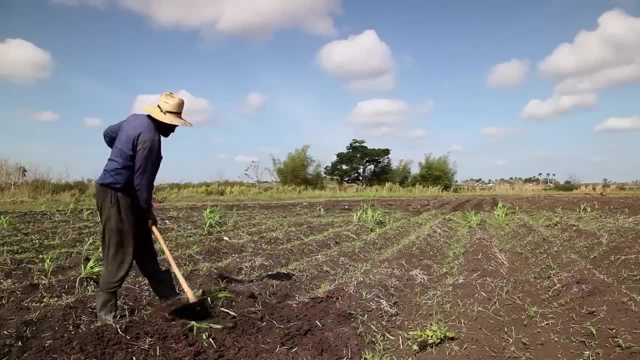 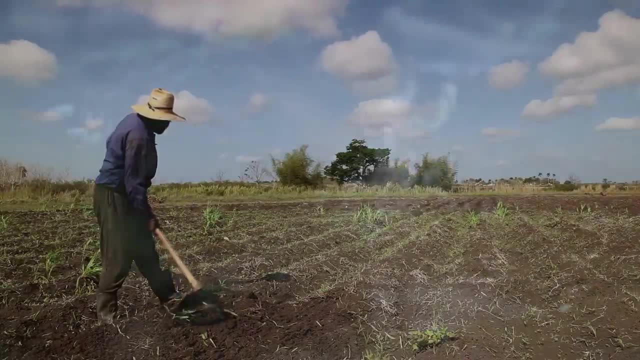 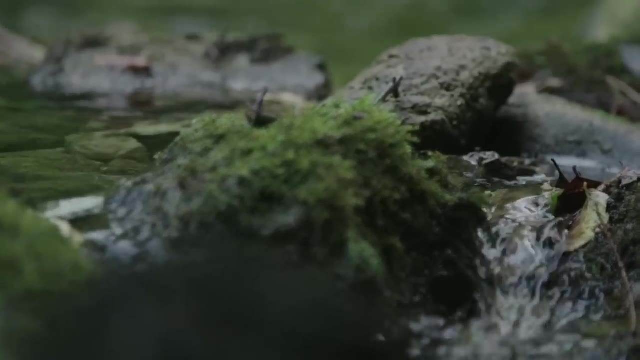 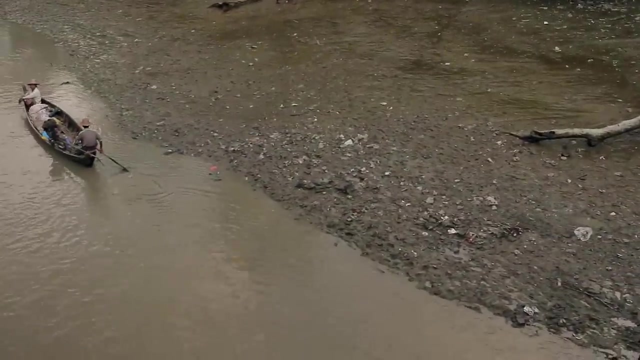 to supply manure to maintain the fertility of farms. Land transport in general was obviously severely limited in the loads and the distances that were possible without animals. Even the navigable waterways were limited in their capacities to move cargo by the absence of make exotic cargoes. when they reached land, Indian canoes plied the inland and coastal. 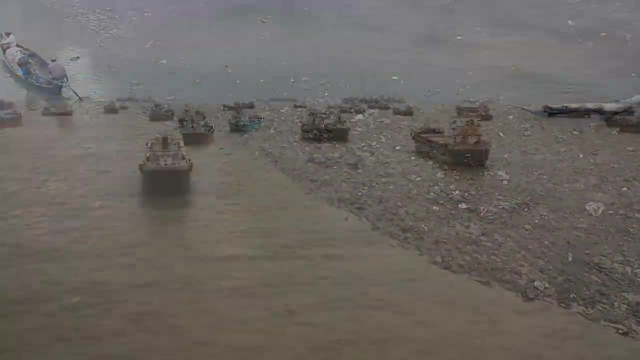 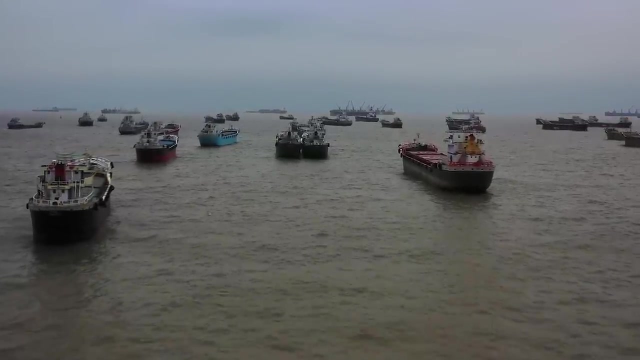 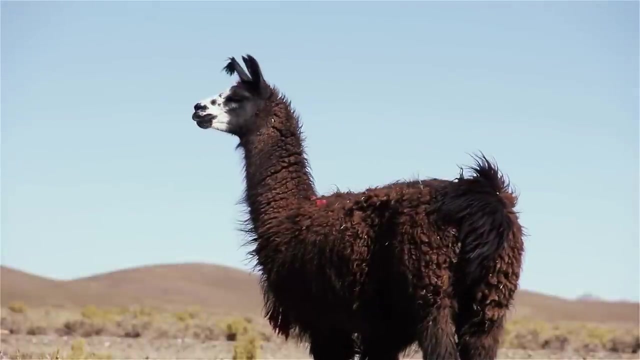 waterways of the Hemisphere long before the white man arrived. but larger vessels with greater cargo capacity would have exceeded the severe physical and economic limits of a land without the kinds of animals needed to make larger cargoes economically viable. Llamas were available as pack animals in limited regions of South America and dogs were used. 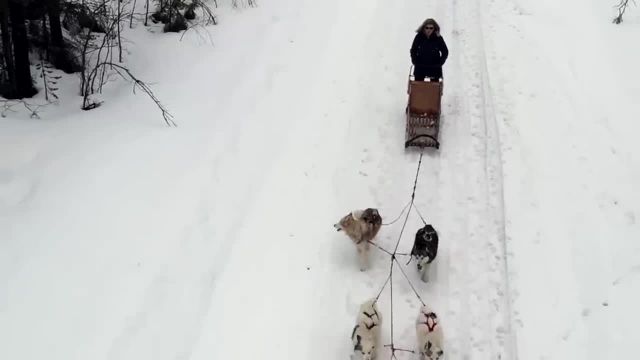 by Eskimos and by some North American Plains Indians to pull loads or to plow the land or to make fewer drifts. Toпons were loaded with 오래 parts and would be required to carry a lot of land so that they could be used for transport. tôpons included Alığımız. 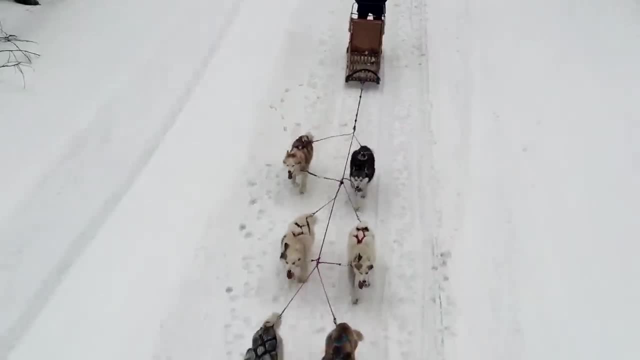 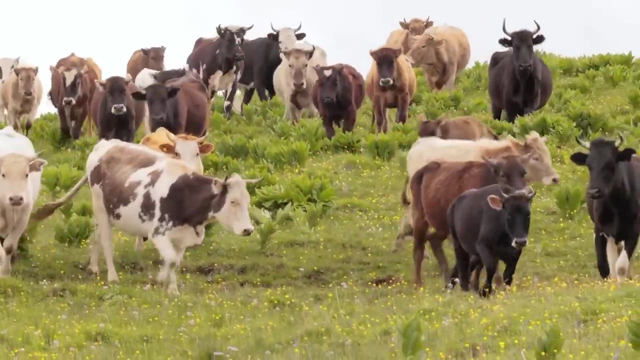 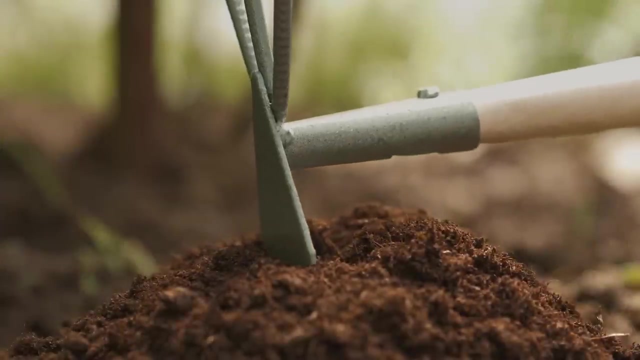 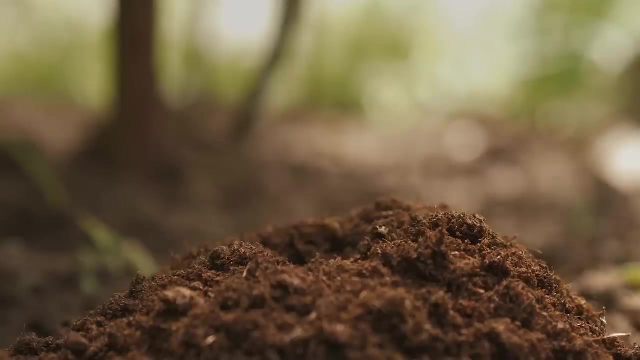 but these animals did not compare with horses or oxen in what they could transport, as in much of sub-saharan africa, not only were loads and distances limited physically in the western hemisphere by an absence of the needed animals, the particular kinds of things that would be economically feasible to trade at considerable distances were even more limited economically to those things whose concentrated value could repay high transport costs, often involving human porters. 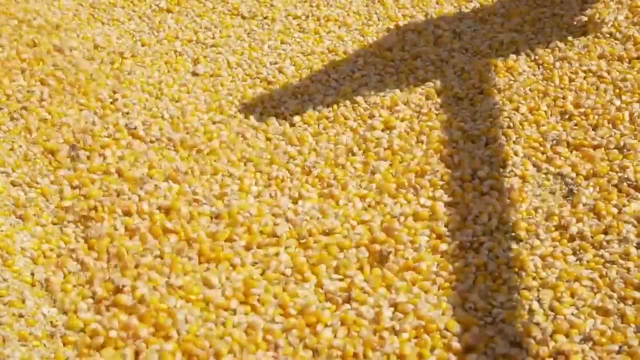 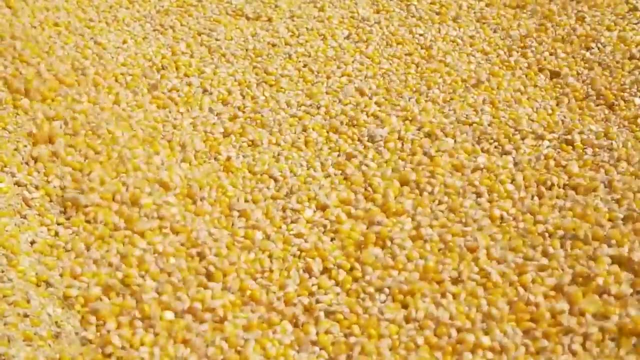 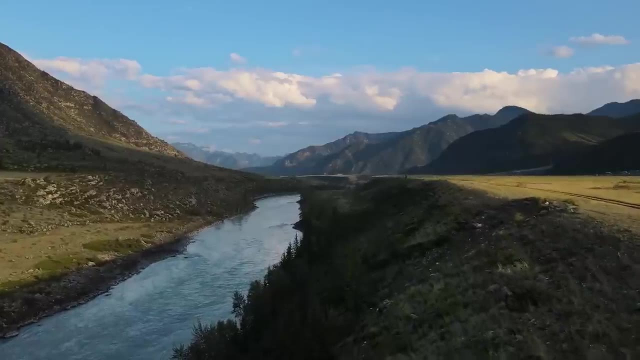 tons of grain, for example, could be shipped for hundreds of miles in europe, but not in the western hemisphere, before the europeans arrived and brought pack animals and draft animals, even in those regions of the western hemisphere that had networks of waterways comparable to those in western europe, limitations on land transport, limited cargoes transported by water. 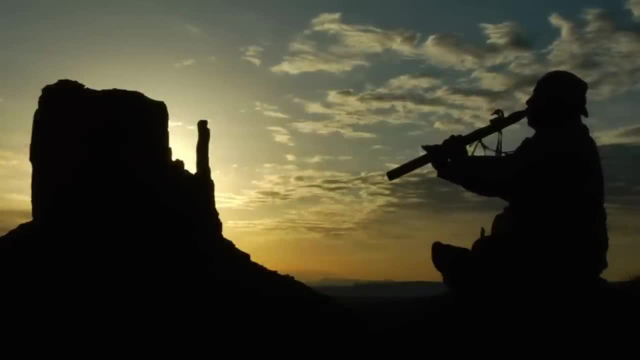 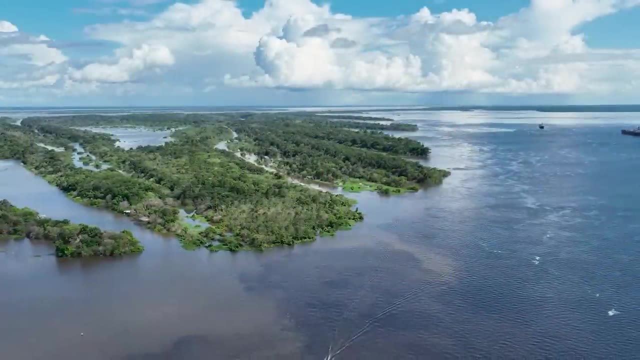 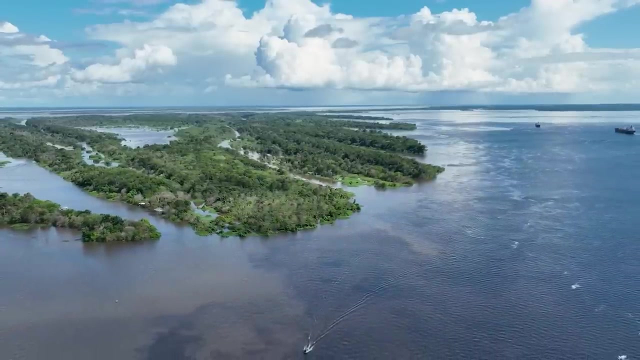 moreover, limitations on the scope and range of trade were also limitations on the scope and range of cultural interchanges. specific geographic barriers- the amazon jungle, the rocky mountains or the vast desert in what is today the southwestern united states- were, of course, major barriers to large-scale cultural interaction in pre-columbian times. 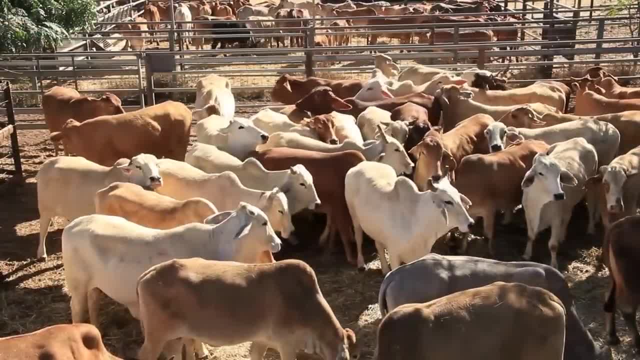 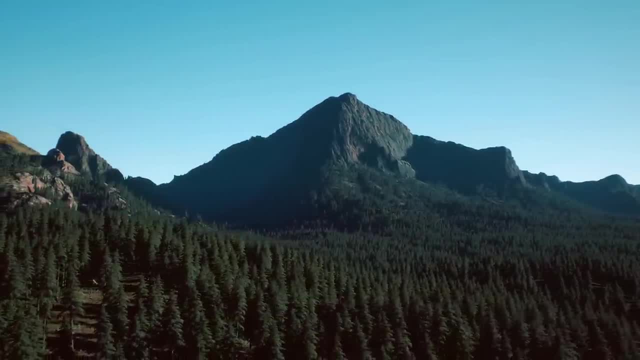 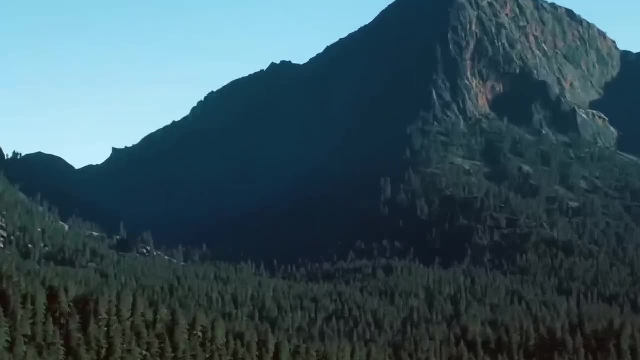 but the absence of animals for transport was a more general barrier to long-range cultural interactions throughout the Americas. While these barriers were not as severe as the geographic barriers in parts of sub-Saharan Africa, they were more formidable than those in much of Europe and Asia. The absence of herd animals like sheep and cattle, as well as the absence of load-bearing or 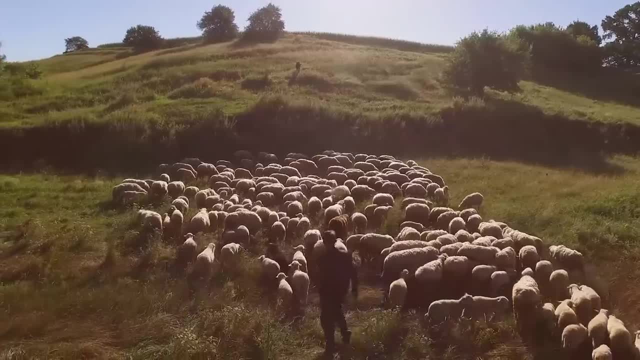 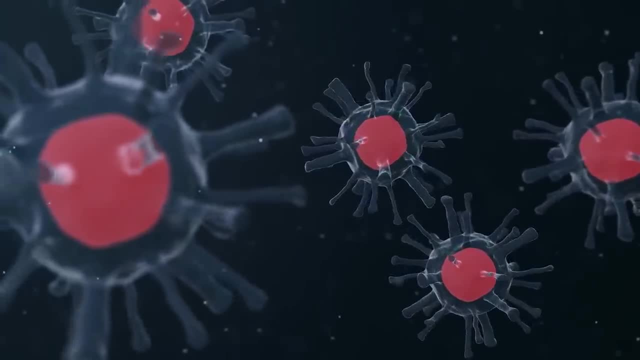 load-pulling animals like horses and oxen had another consequence—an absence of the many diseases carried by such animals and often acquired by human beings living in close proximity with these animals. While, in one sense, the absence of such diseases was, of course, a 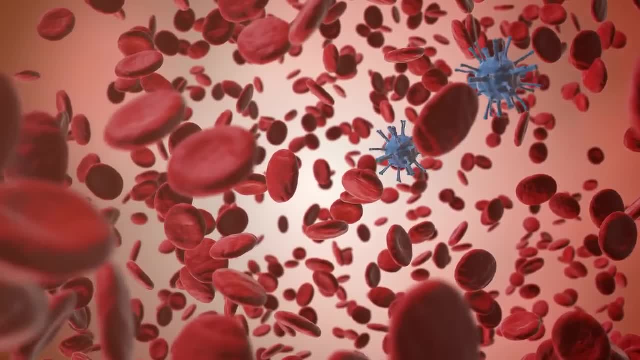 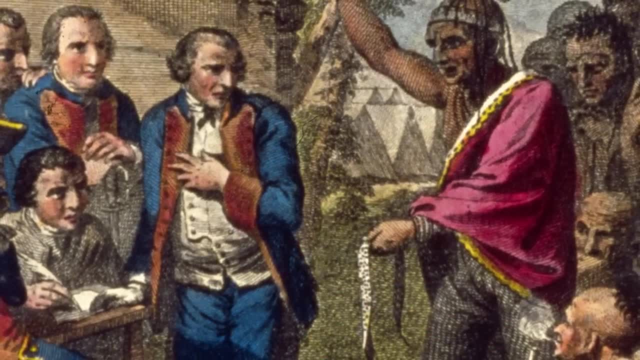 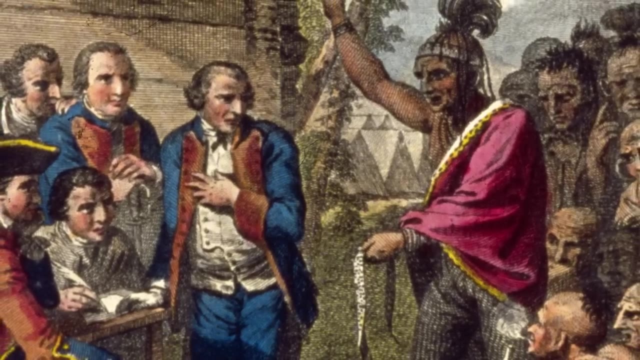 benefit. their absence also meant an absence of biological resistance to many potentially devastating diseases such as smallpox. So long as such diseases did not exist in the Western Hemisphere, the Indians' lack of biological resistance to them was of no consequence. But once people from Europe 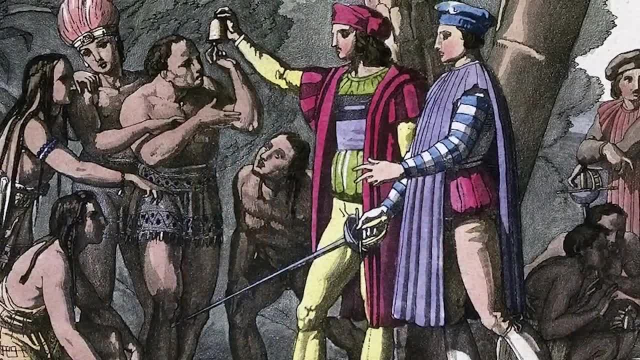 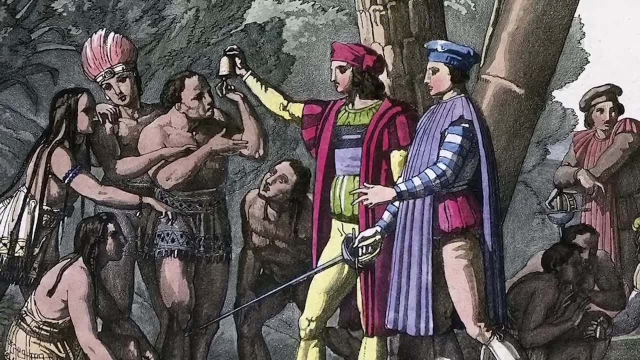 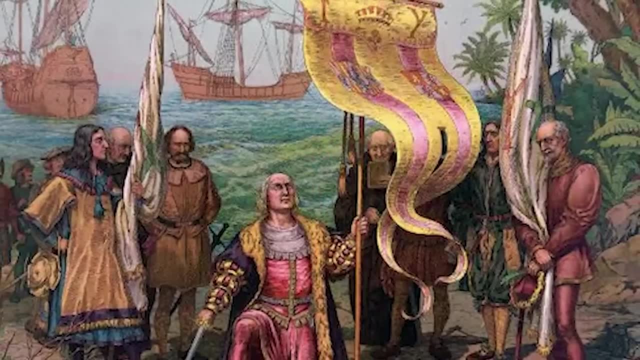 began arriving with these diseases. the consequences were momentous, not only for those indigenous populations stricken and devastated by these diseases at the time, but also for the historic transfer of North and South America from the indigenous peoples to the European invaders. The most invincible of these invaders proved to be not the Europeans themselves. 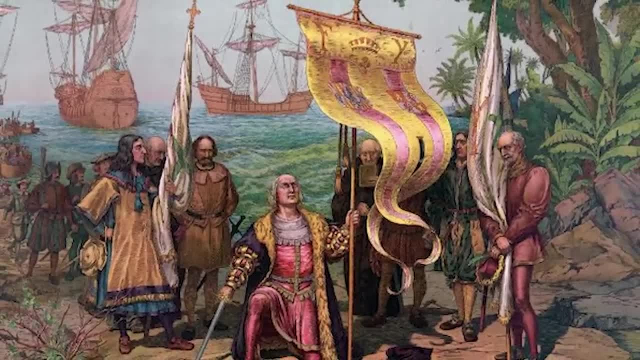 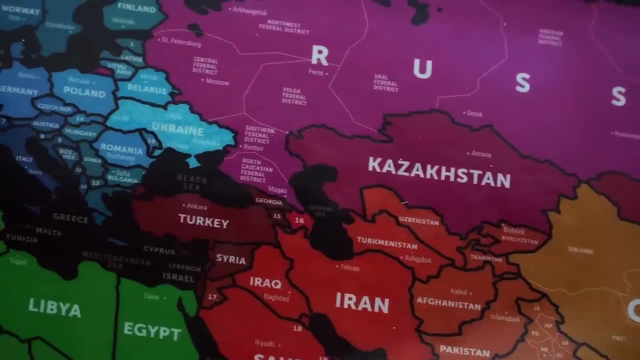 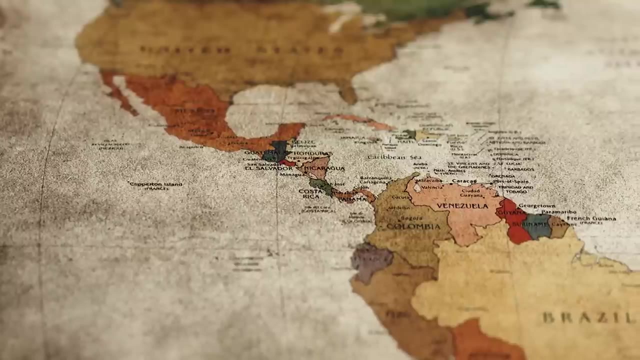 but the invisible carriers of their diseases, whose existence neither they nor the Indians suspected. The fact that the Eurasian landmass stretches predominantly east and west, while the Western Hemisphere landmasses stretch predominantly north and south, means that advances in agriculture and animal husbandry could spread more readily over far more distances in the Old World than 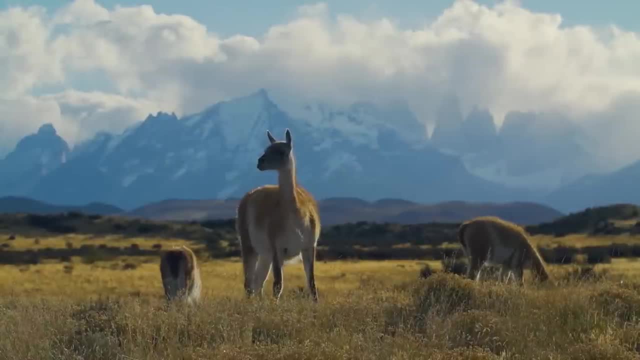 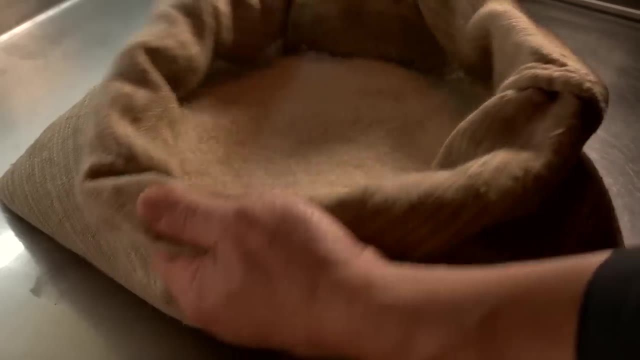 in the New. Plants and animals are more similar in the same latitudes, while more drastic climate changes accompany North-South movement. Thus rice cultivation could spread across Asia, to Europe and ultimately to North America, But by the end of the 20th century the population 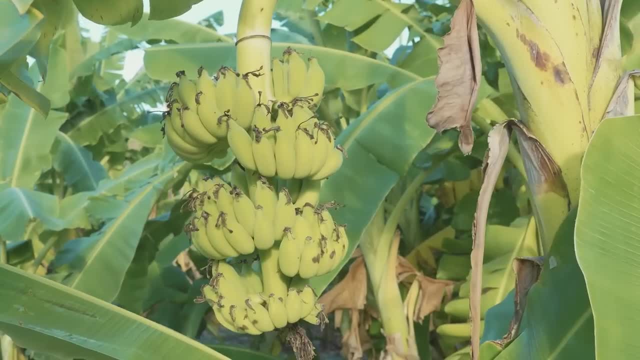 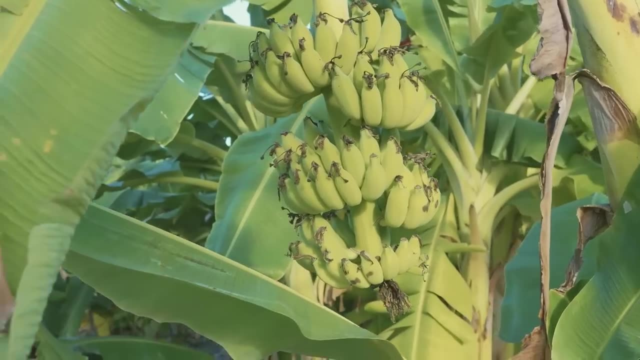 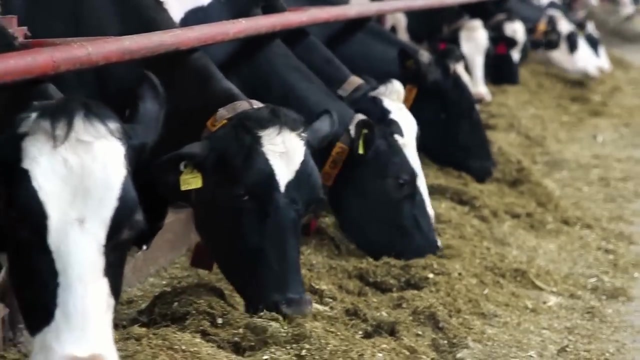 would have been reduced to only a little With the rise of the economic growth. the population would have been reduced to less than a third of what it was before the war. But in the but bananas could not spread from central america to canada, nor could many of the animals adapted to the tropics survive in the colder climates to the north or south, so that knowledge of how to hunt or domesticate these animals was similarly restricted in how far it would be applicable. 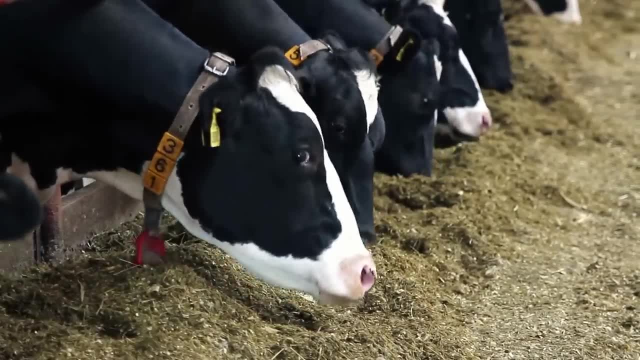 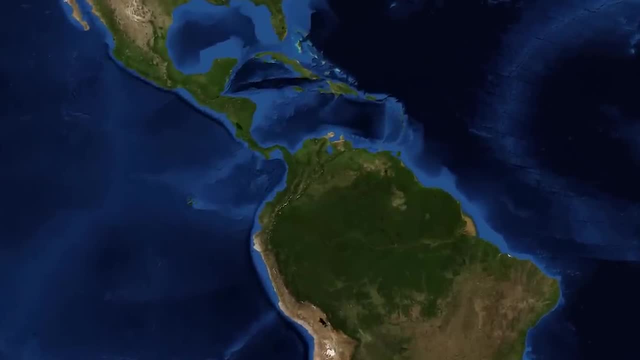 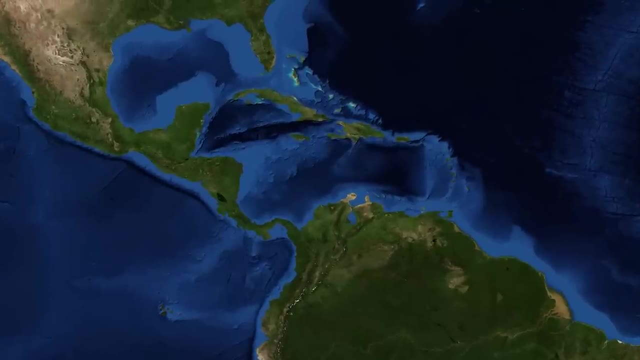 even if such knowledge could be transmitted over long distances. moreover, the northern temperate zone and the southern temperate zone of the western hemisphere were too far apart to make any sharing of knowledge between them feasible in pre-columbian times. in short, climate, like other aspects of geography, limited the size of the cultural universes of the indigenous peoples. 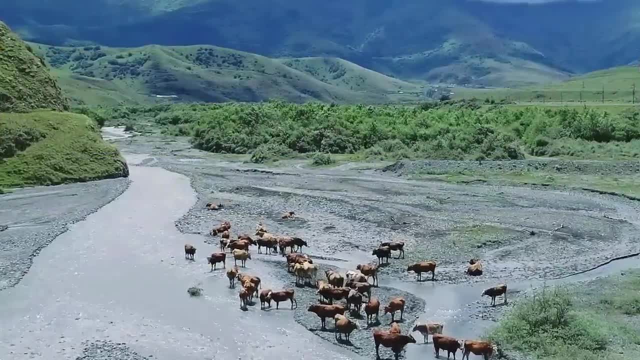 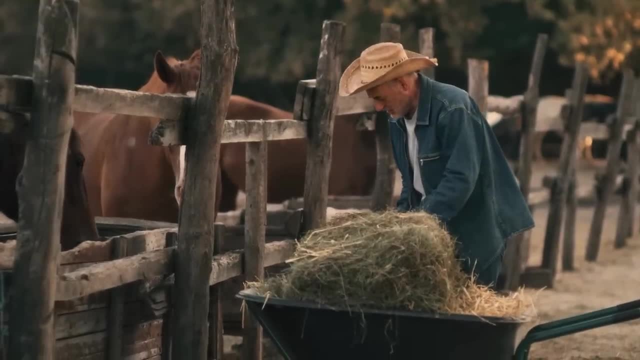 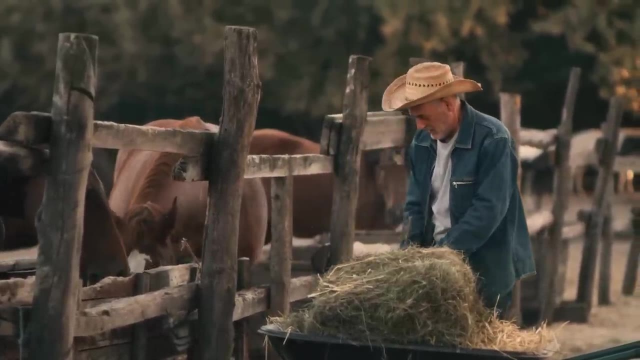 of the western hemisphere. the geographical environment of the western hemisphere itself changed with the european conquest. vast herds of new animals were transplanted from europe, along with the invisible transplanting of a whole new disease environment and a whole new technology from europe. these transplantations 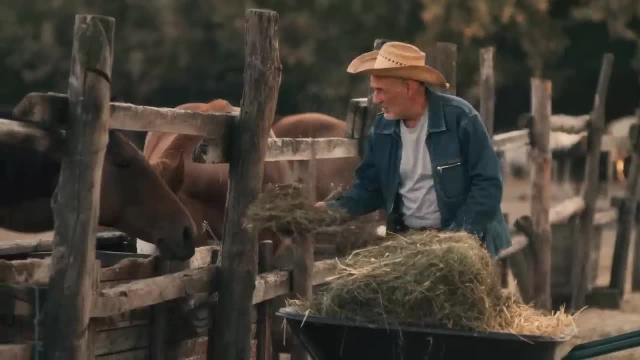 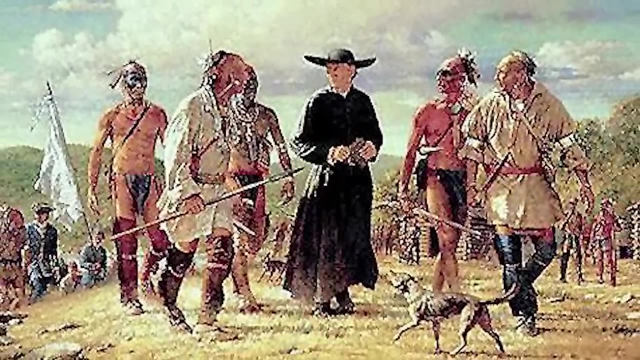 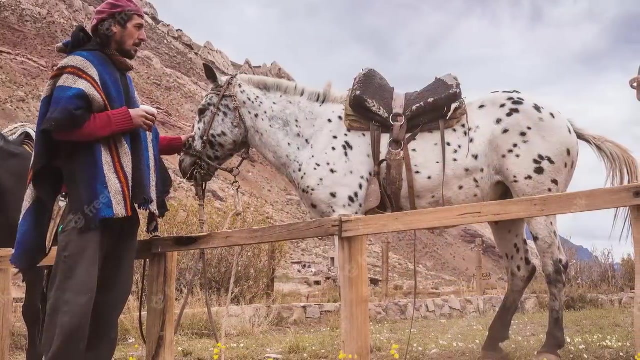 changed the lives of the indigenous peoples, as well as allowing the european settlers to bring much of their cultural world to the americas. mounted indian warriors with herds of cattle became a traditional way of life on the western plains of the united states, for example, while the gauchos, who herded cattle for spanish 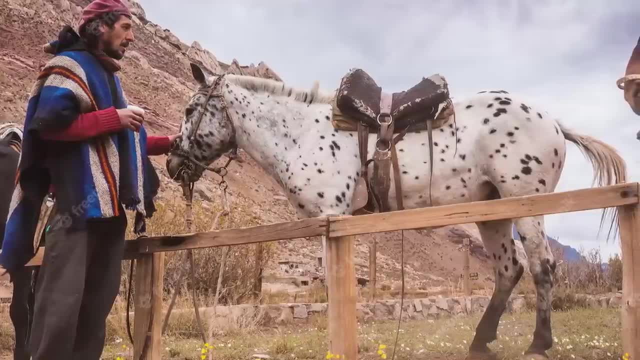 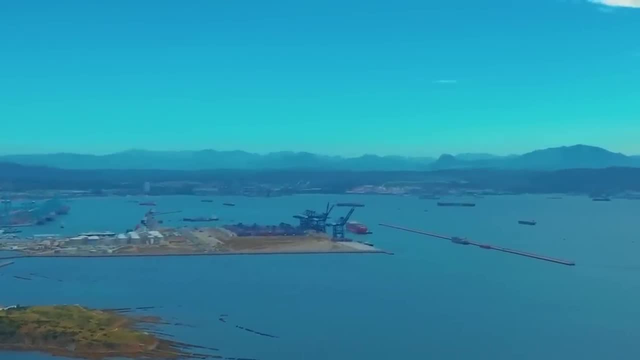 landowners on the argentina pampas were often part or full-blooded indians as well. such physical features of the western hemisphere as natural harbors and rivers reaching deep inland from the sea now became far more important economically after the arrival of white invaders. 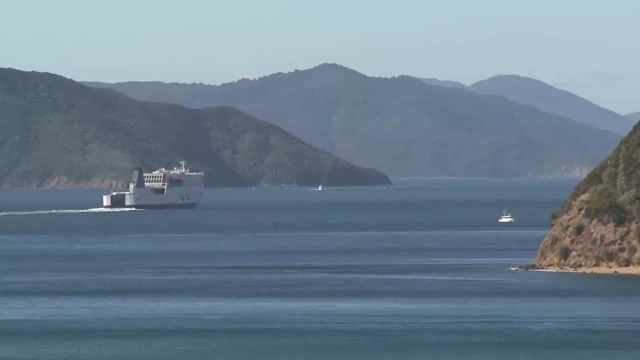 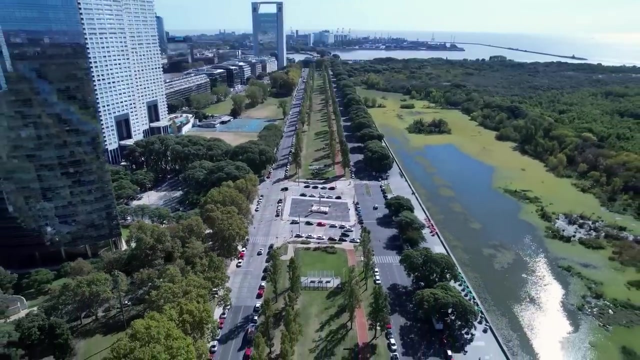 and settlers in ships developed in europe but better adapted to exploit new world conditions than were the canoes of the indians. those parts of the western hemisphere most highly developed by the europeans were not the same as the indian peoples who were brought to the western hemisphere. 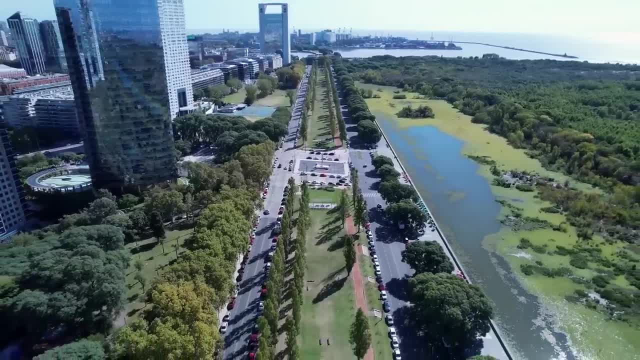 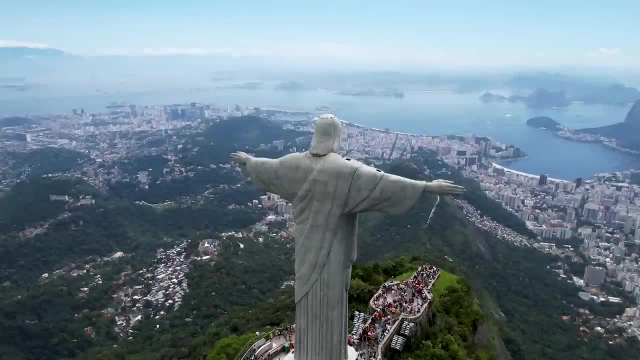 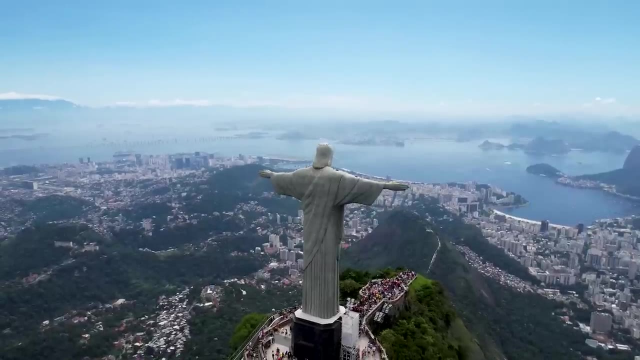 as those that had been most highly developed by the indigenous peoples. whereas the most advanced indian civilizations developed in central america and in the andes mountains, the most advanced regions developed by europeans were those regions whose geography was most like that of western europe: places with natural harbors and broad coastal plains. 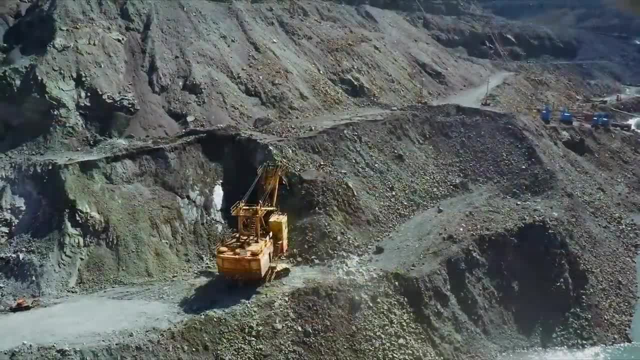 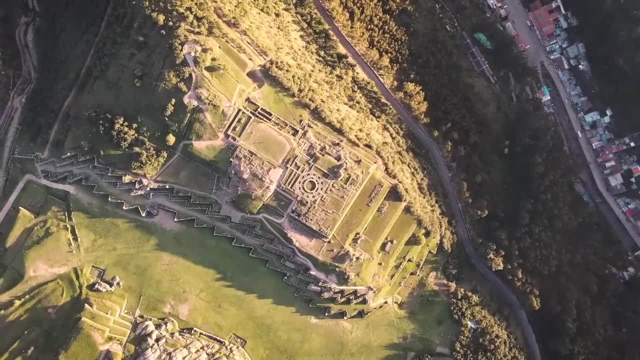 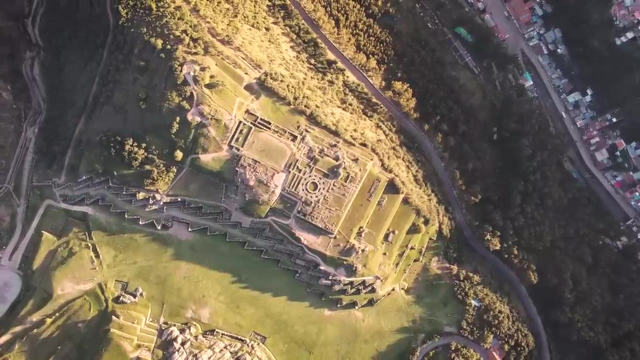 criss-crossed by rivers deep enough to carry large ships and, eventually, places with the mineral deposits needed to build an industrial society. Only in the narrowest physical sense was the geographic setting of the Western Hemisphere the same for the indigenous peoples and for the Europeans, The flora, the fauna and the disease. 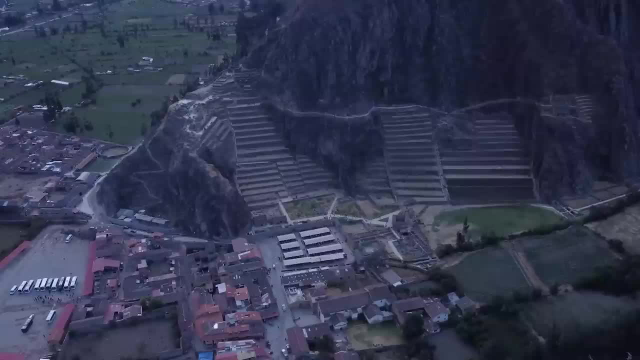 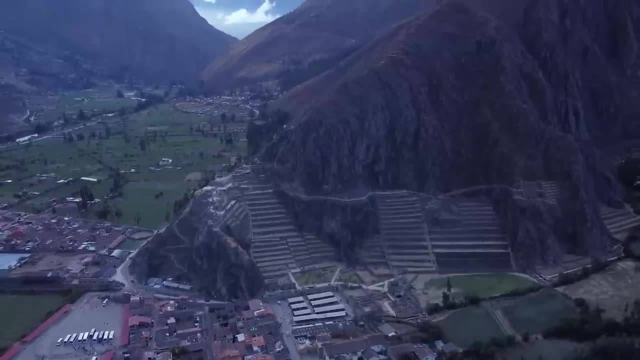 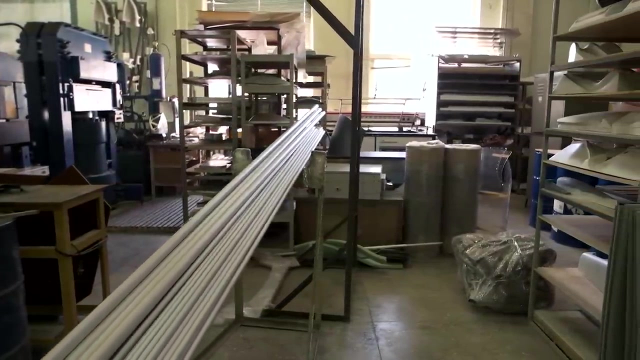 environments were changed radically and the natural features of the land and the waters acquired a much wider range of possibilities as a result of this, as well as because of the new technology brought from Europe. Moreover, the technology that the Europeans brought to the Western Hemisphere was not simply the technology of Europe. Because of the geography of the Eurasian 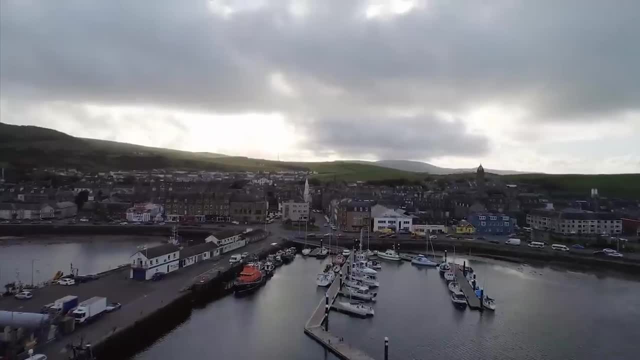 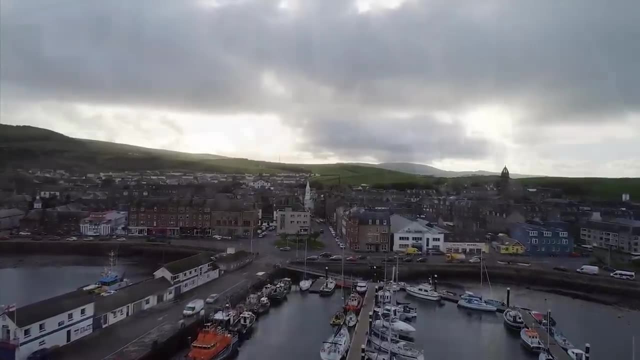 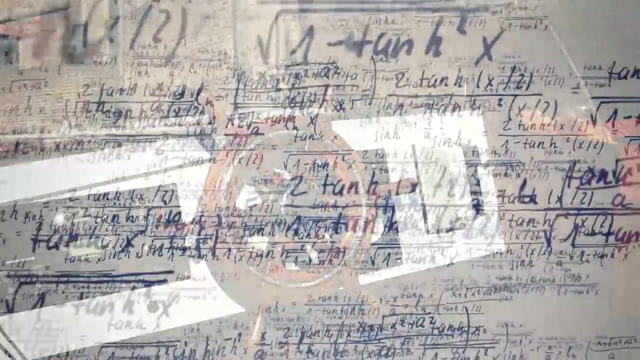 landmass. Europeans were able to bring to bear in the Western Hemisphere the cultural features of lands extending far beyond Europe, but incorporated into their civilization. Europeans were able to cross the Atlantic Ocean in the first place because they could steer with rudders invented in China, calculate their position on the open sea through trigonometry. 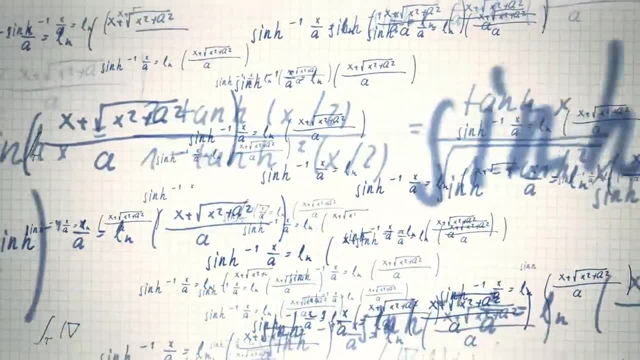 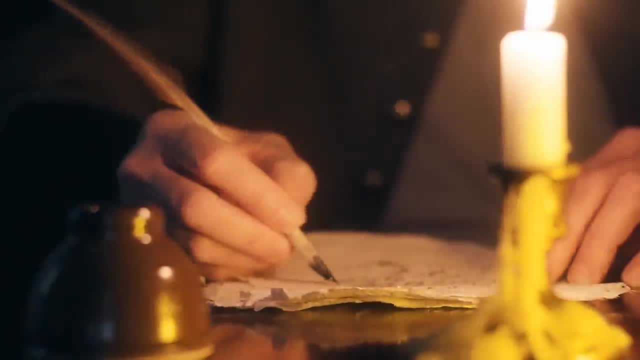 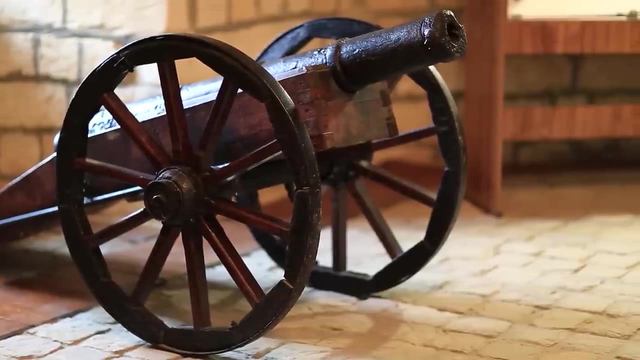 invented in Egypt, using numbers created in India. The knowledge they had accumulated from around the world was preserved in letters, invented by the Romans and written on paper invented in China. The military power they brought with them increasingly depended on weapons using gunpowder, also invented in Asia. 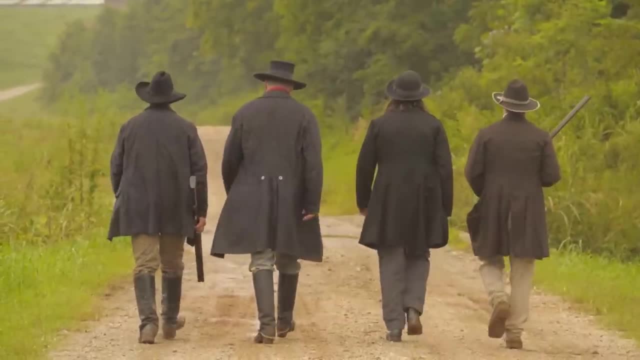 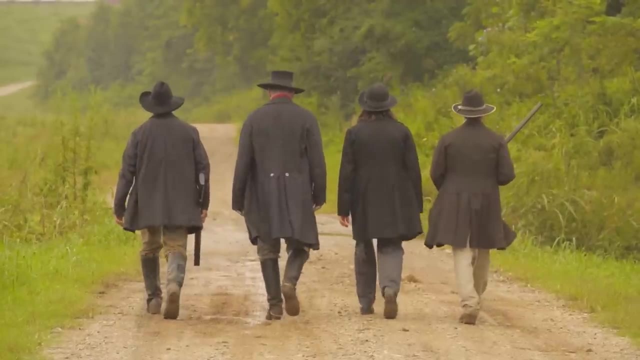 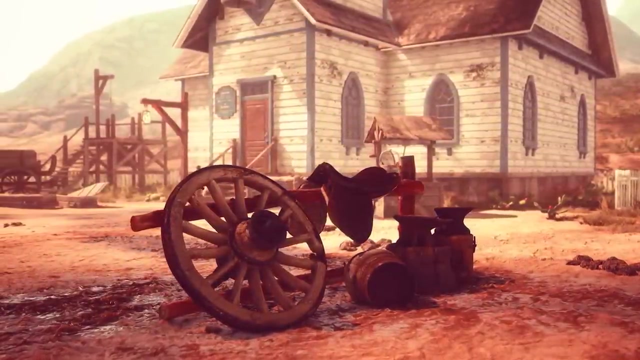 The cultural confrontation in the Western Hemisphere was, in effect, a one-sided struggle between cultures acquired from vast regions of the earth against cultures from more narrowly circumscribed regions of the New World. Never had the advantages of a wide-ranging intercultural universe been more dramatically or more devastatingly demonstrated than in the conquests that followed.